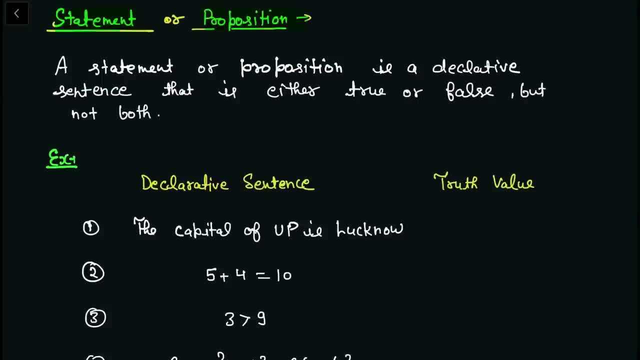 So if we talk about a statement or proposition, A statement or proposition is a declarative sentence. What is a statement and a proposition? What is a declarative sentence? A declarative sentence, sentence. That is either true or false. 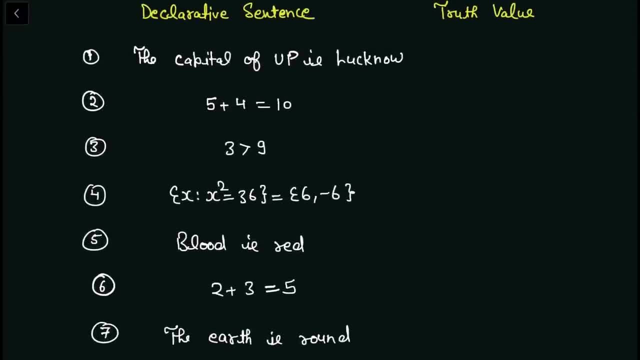 That is what defines our statement or proposition. For example, I will take some examples of statement or proposition. 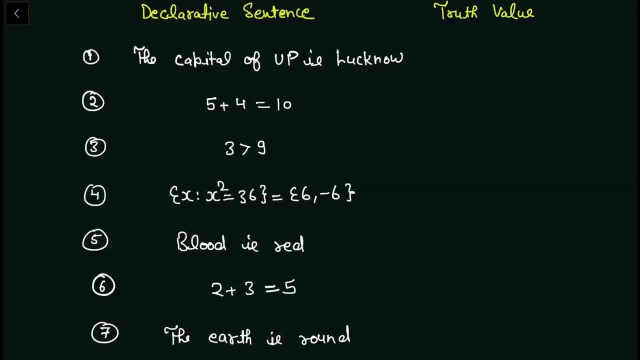 On one side, I will write a declarative sentence and on the other side, we will check if it will take true value or false value. Truth value, which we call. 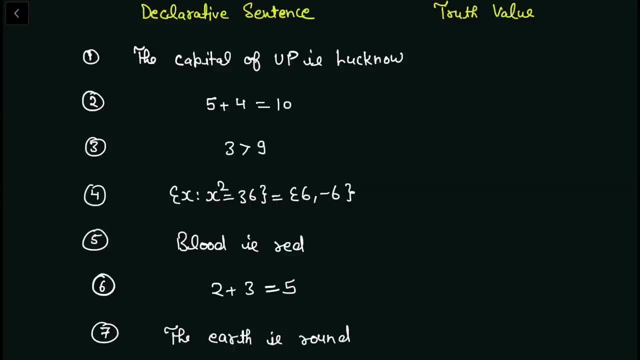 So, the first one is the capital of UFP is Lucknow. You know that this statement is true, right? So, here it will take true value, which we can call T. So, 5 plus 4 equal to 10. Does 5 plus 4 equal to 10? No, it is not true. 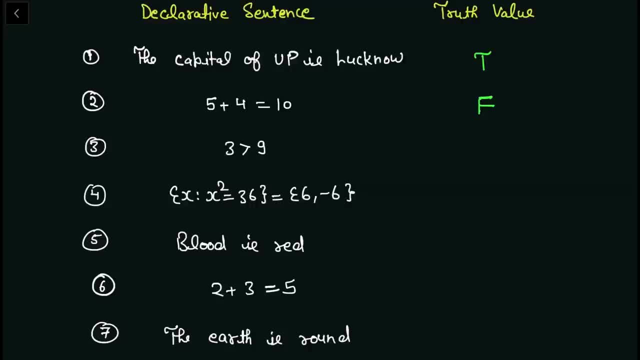 If it is false, then it is a false statement. 3 greater than 9. 3 can never be greater than 9. So, this is also our false statement. 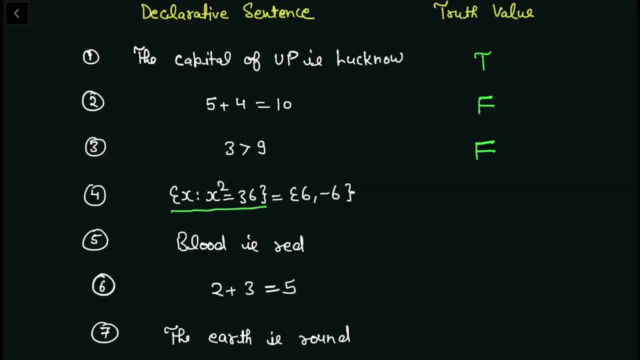 Then, our condition is x is a set in which x square is equal to 36. Then, here it is written equal to 6 minus 6. So, you know that if we keep the value of x as 6, then also 36. That means, the condition will be satisfied. If we keep minus 6, then minus 6 square will be 36. 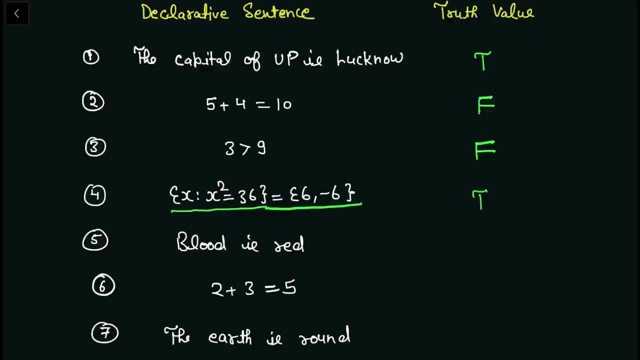 Then also, the condition will be satisfied. That means, this statement, this declarative sentence, this is also our true. Declarative sentence, either it will be true or false, both will not happen. 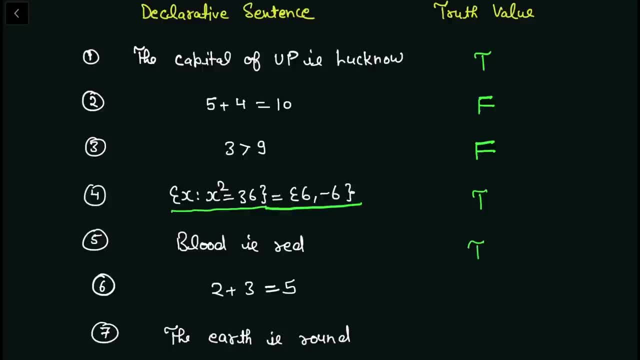 Blood is red. You know that statement is our true. So, it will take true value T. 2 plus 3 is 5. True value T will take. As if the earth is round. 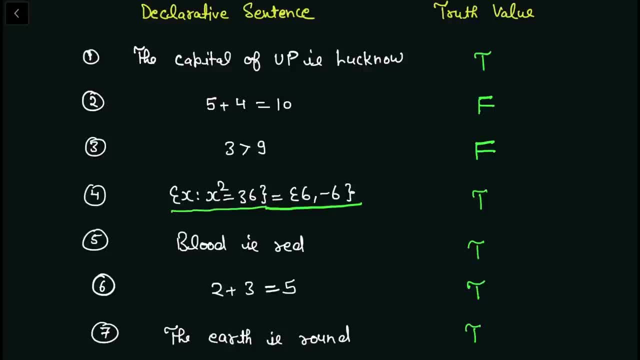 This is also our statement, declarative sentence. This will also take our true value, T. So, declarative sentence either it will take true value or false value. Both values will never take together. Okay. 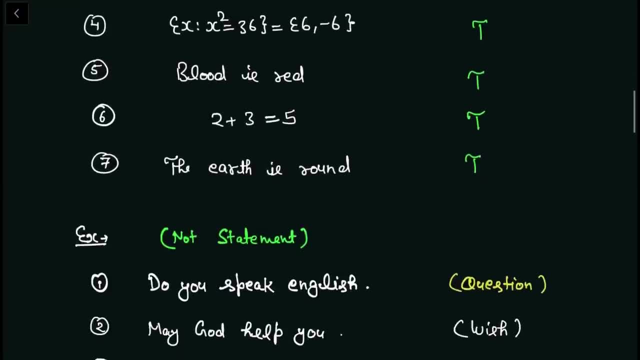 So, I have told you some examples which are of proposition or statement. Right. 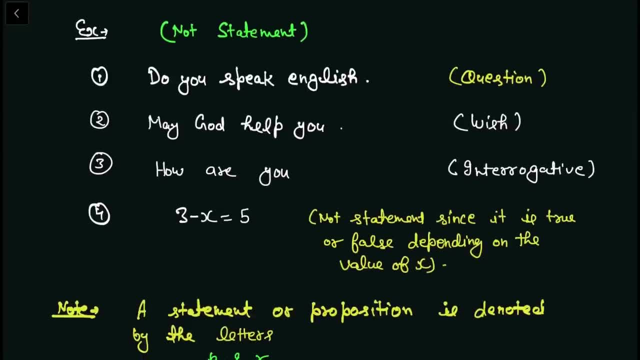 You can cover yourself from the rest of the book as well. I will take some examples which will not make statement or proposition. 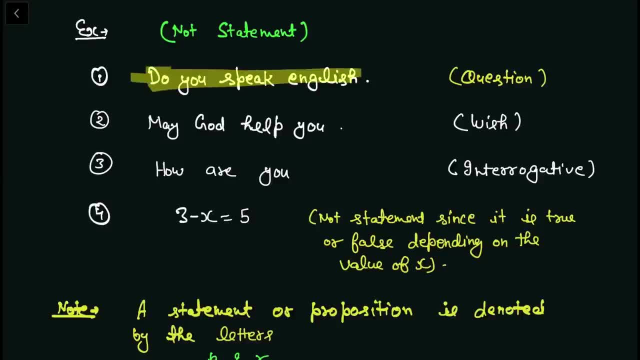 For example, like a sentence is written here. Do you speak English? So, you can see that this is our question. 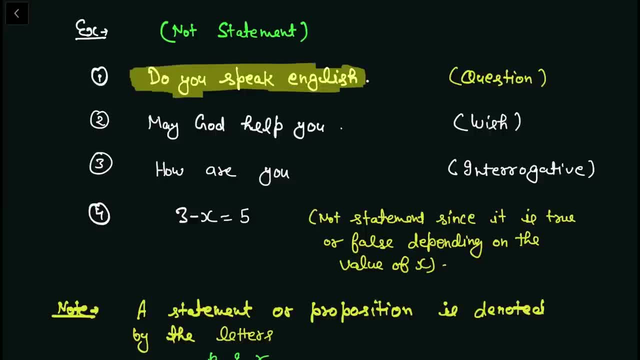 We will never call this statement. This is not a statement. This is a question. The question has been asked. Do you speak English? May God help you. May God help you. This also will not make any sentence or statement. Because this is a wish. How are you? How are you? This is also a question. 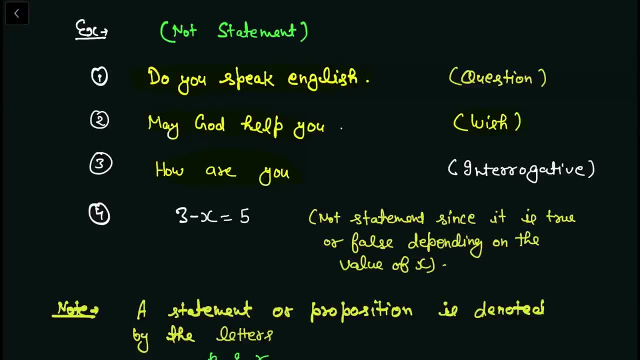 This is an interrogative sentence. This will not be a declarative sentence. So, this also will not make our statement. 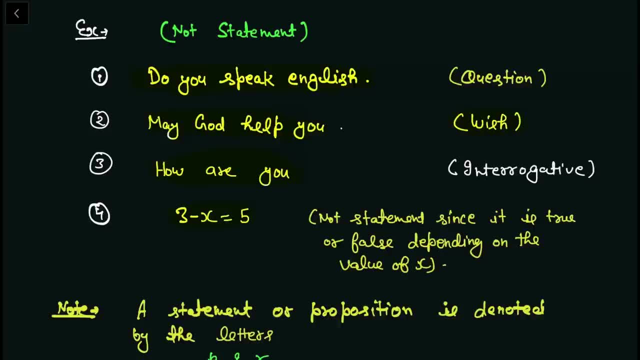 Three minus X equals to five. This is also not our statement. 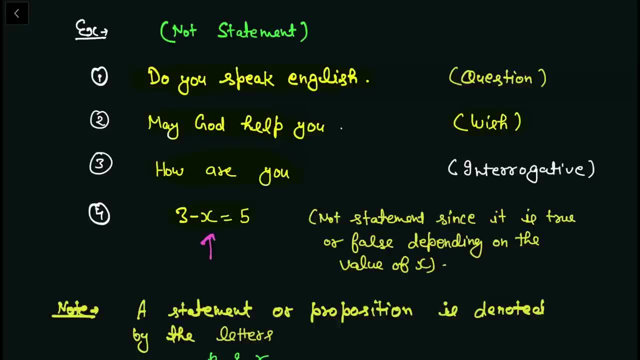 Because this condition will be true or false. How does this depend on X? 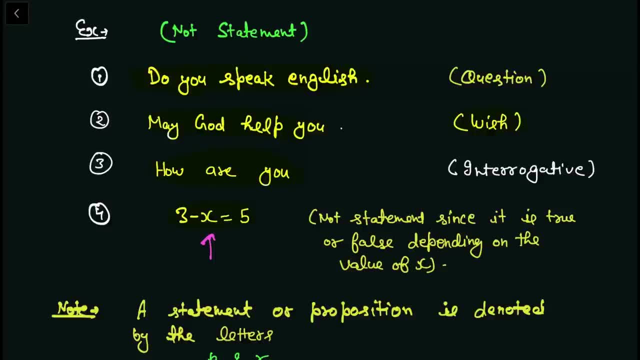 If we took X's value as two, then you will get some other value. If you took 3, then you will get some other value. It can be true or false. 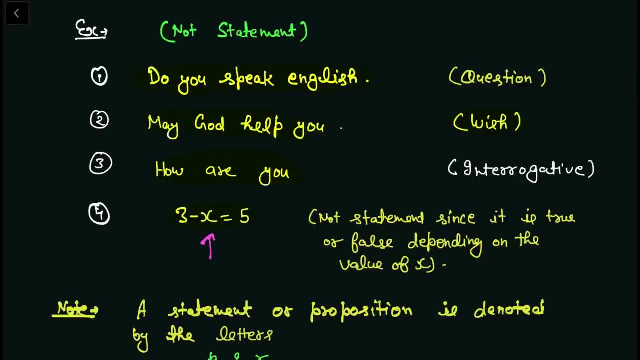 If you take X's value as minus eight, it will be true. If you take X's value as plus eight, it will be false. 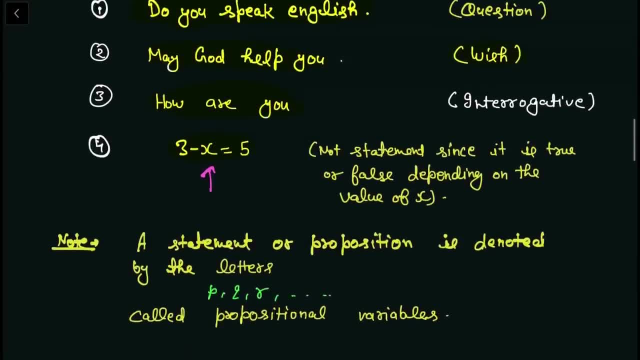 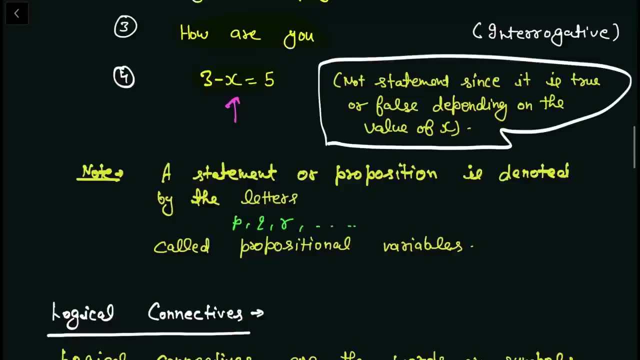 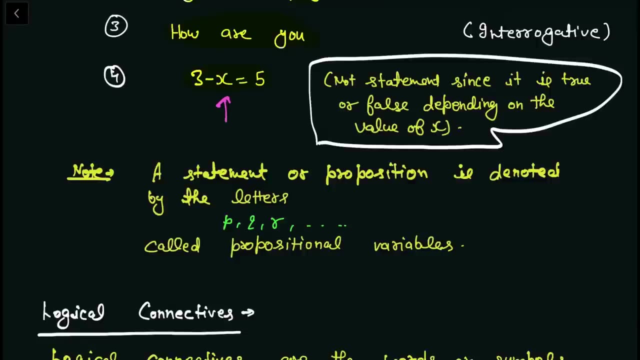 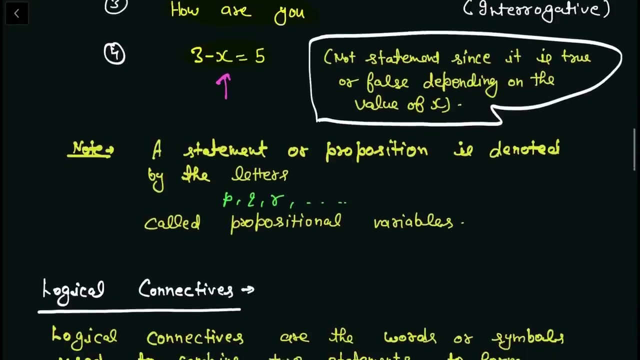 So, this depends on X's value. true or false so this is not a declarative sentence this is not a statement so this is not a statement or a proposition so I told you some examples in which I told you some conditions of statement or proposition that any declarative sentence which takes true value or false value will be a statement and if someone can take both values or if there is uncertainty then we say that it is not our statement or proposition 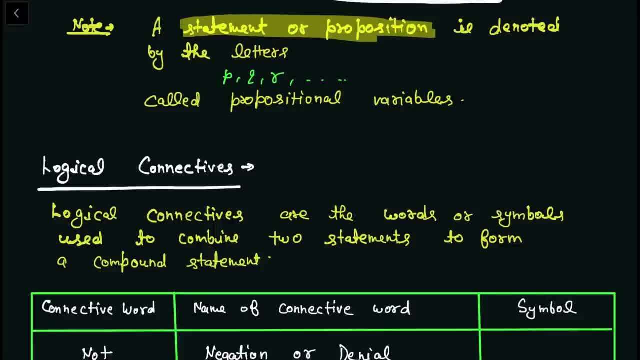 always remember that we will use the notation of proposition or statement in module 4 we will use it in this way we will denote statements from P, Q, R, S in this way we denote in PQR and all these variables we call them variables related to proposition which we will name as propositional variable PQR is a statement which is our propositional variable 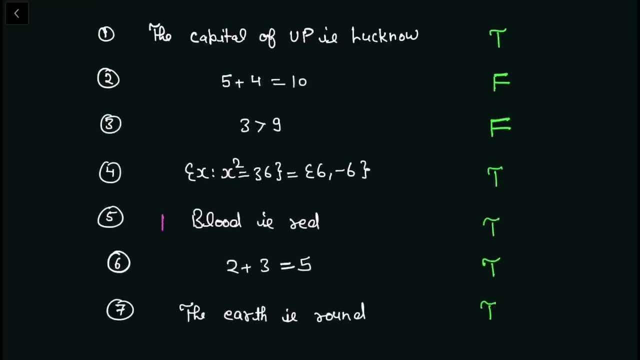 like how we will define PQR like blood is red this is our sentence 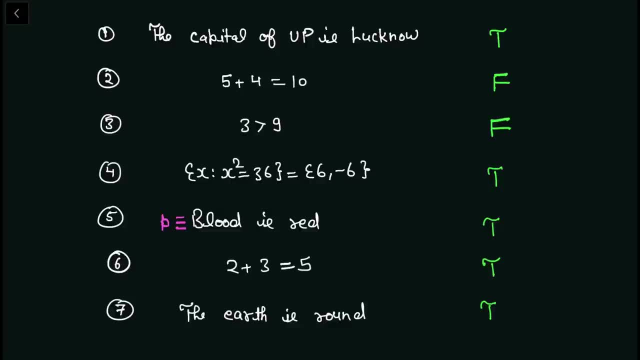 so we will name it as P and like our second sentence is 2 plus 3 equal to 5 we will name it as Q so in this way we can name 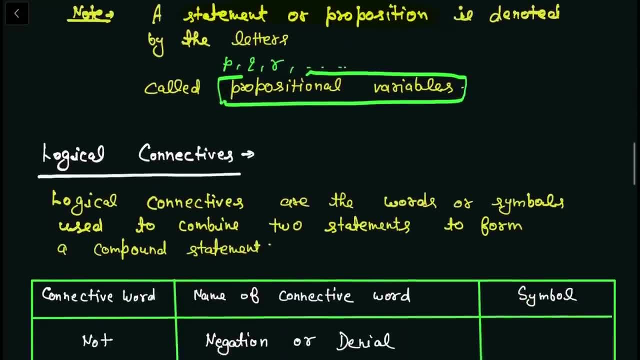 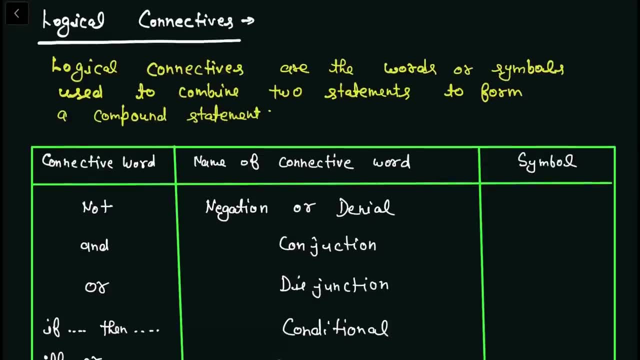 any sentence as a variable in the form of PQR we call them propositional variable now this is our statement or what is a proposition and how we can tell true value or false value 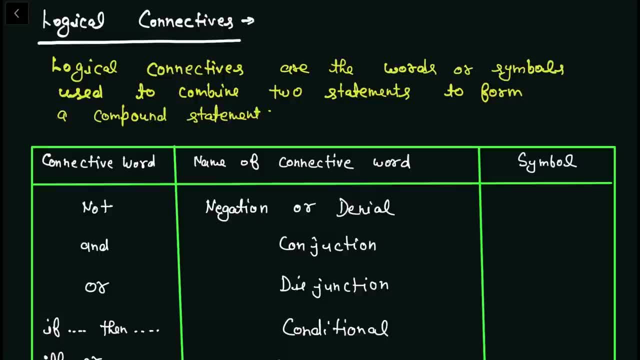 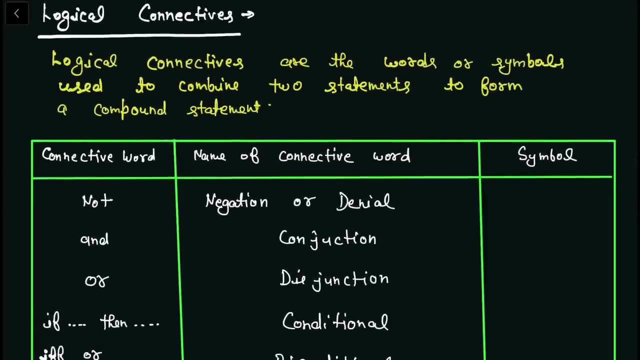 now any two statements or more than two statements we can operate in each other means in that we can make some logical connection and the logical connection which we make here basically we use five types from which compound sentences are formed what are they we discuss them logical connectives are the words or symbols 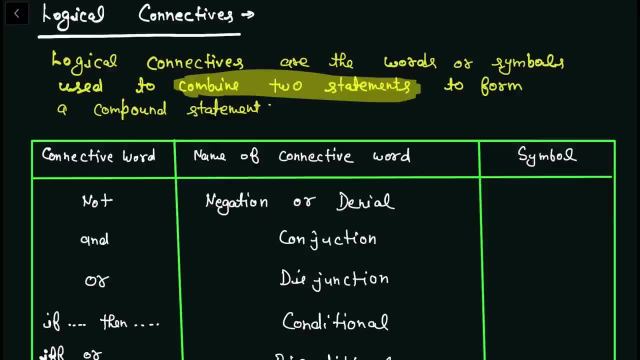 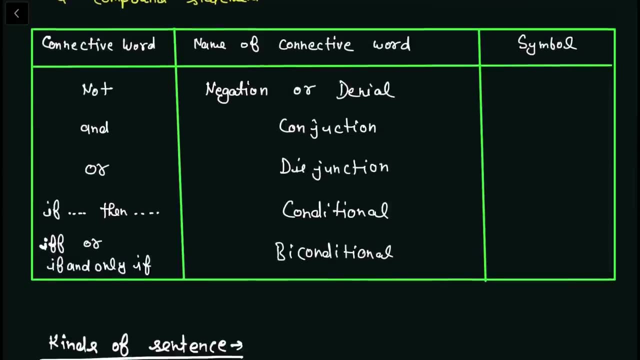 which we use as logical operators use as logical connectives so that our statement can be compounded compound means combine so they will go in logical connectives logical connectives means we will define some operations first of all our connective word if we have a note so for note the operation we define we call it negation name of the connective word 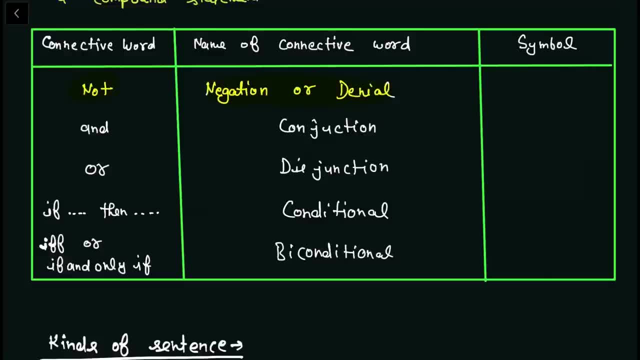 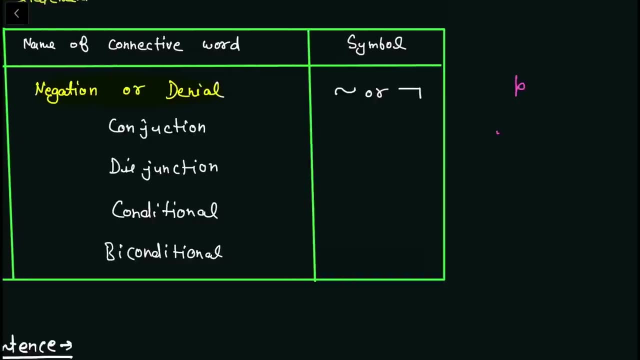 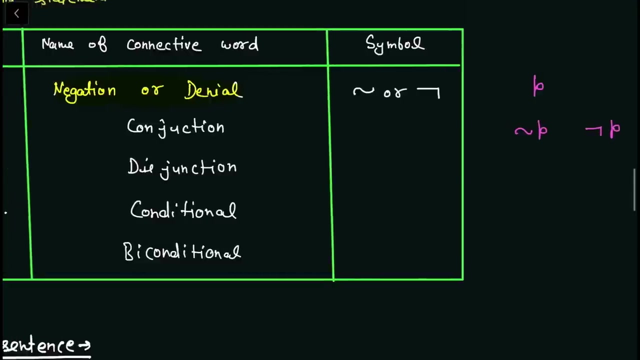 or sometimes it is also called Daniel and for note the symbol we use one of the two symbol can be used in exam either this symbol or this symbol both of these symbol are used for note for example if p is a statement then negation of p you will write note p or you will write note p ok so you will write negation of any statement ok for example we gave name to p we gave name to p the earth is round we gave name to p 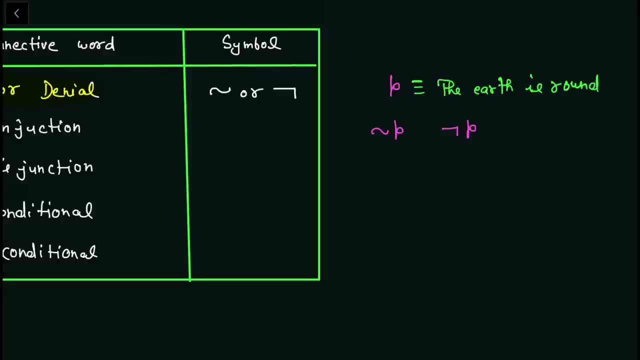 the earth is round so what will be its negation 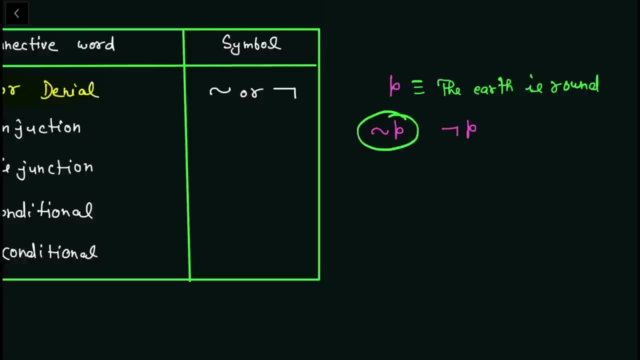 what will be its reverse what will be its reverse the earth is not round 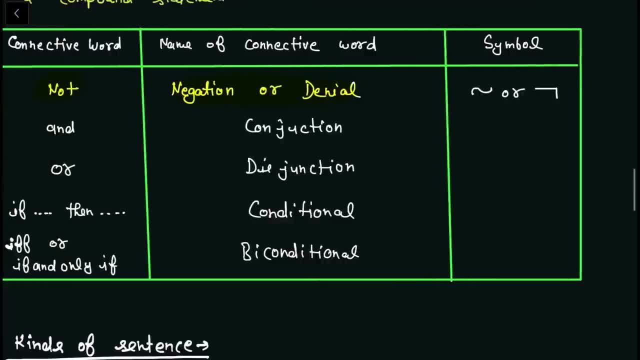 we will give name to negation p negation p note p ok so for note word 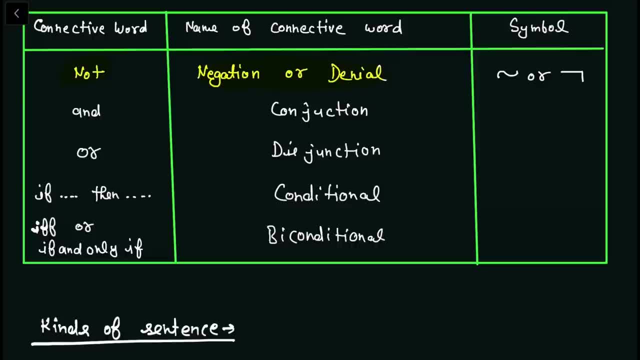 we use negation which is our first operation for statement second operation is end operation ok 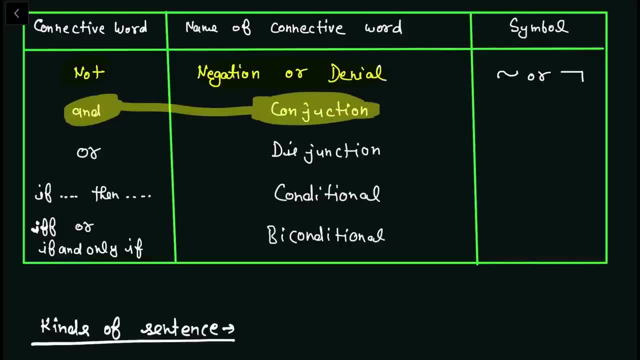 second operation is end operation and for end 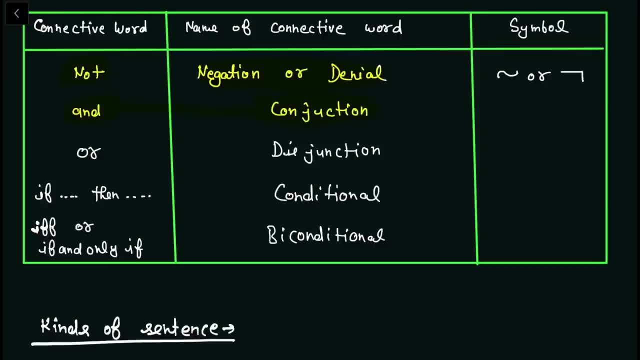 the connective word we use is conjunction and conjunction is nothing meet which you have read in module 3 meet is called conjunction 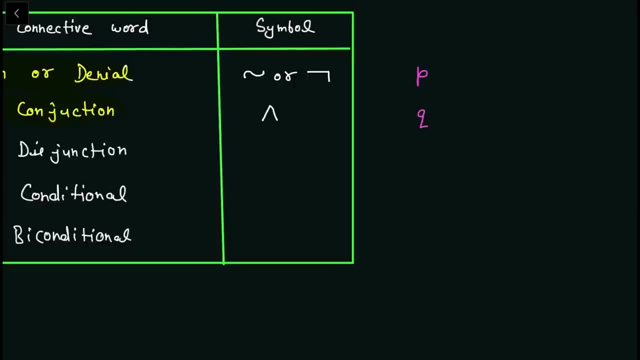 and we use conjunction for end for example we have two statement p and q so if we write p meet q it means p conjunction q and this word is used for end for example if end comes between two statement then we can use conjunction ok we can use conjunction for example p statement pi is greater than 3 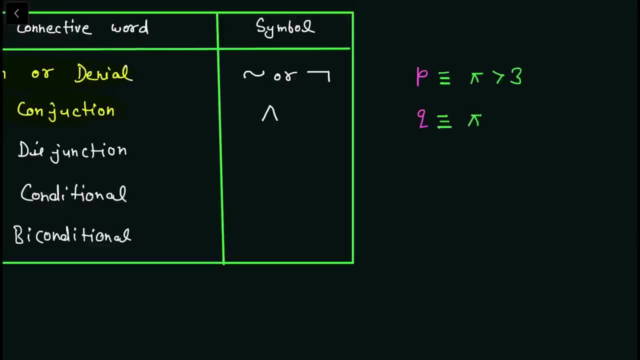 q statement pi is less than pi is less than 4 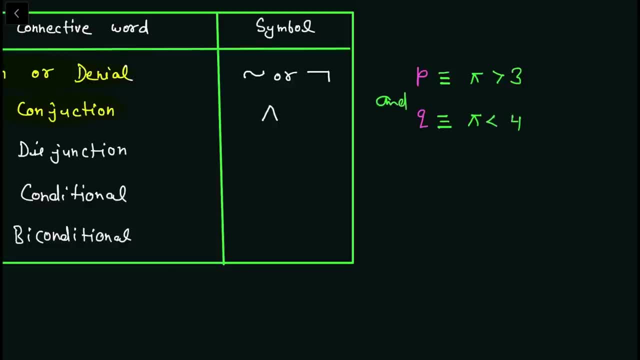 ok so we can use end word p and q 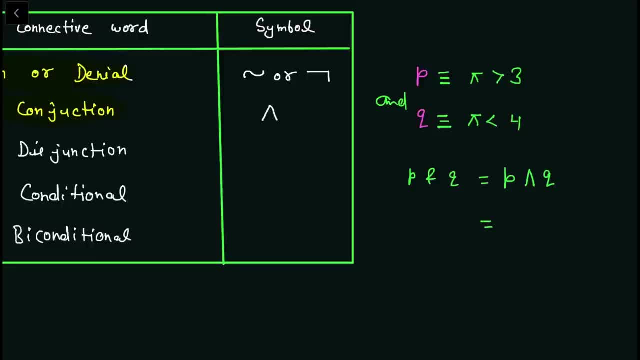 p conjunction q p conjunction q 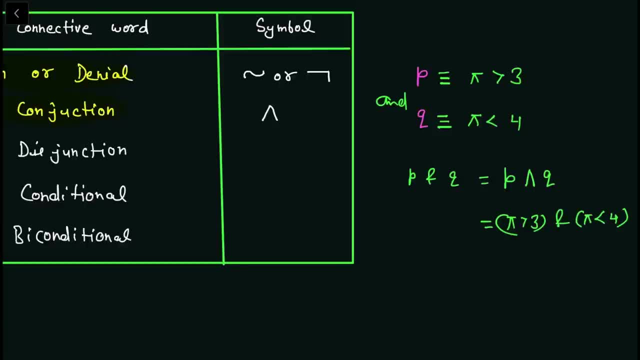 pi greater than 3 and pi less than 4 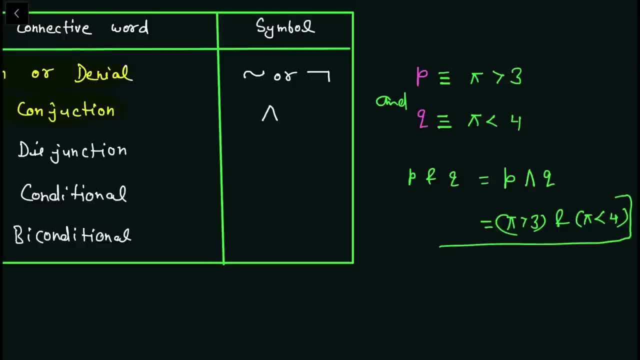 so if we use end word to combine two propositions then p conjunction q 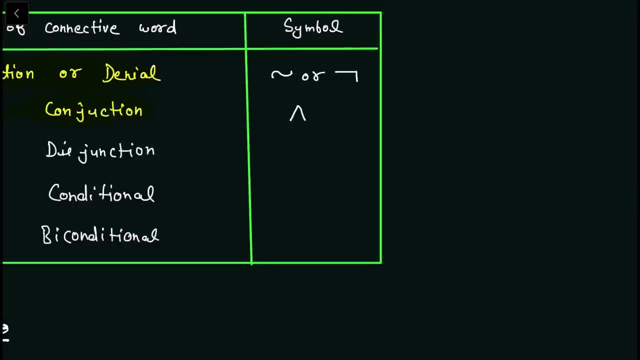 ok and for conjunction we use meet k 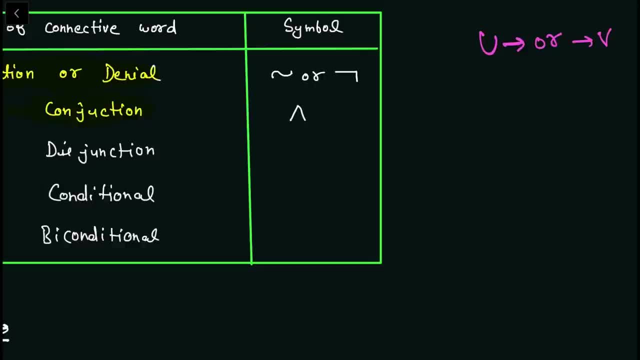 like you have read in set theory union we use or k 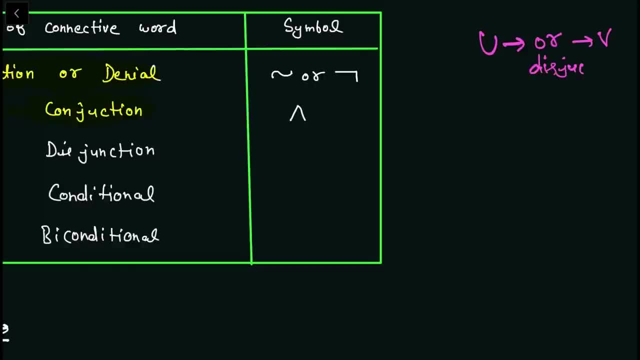 so for union we use join operation 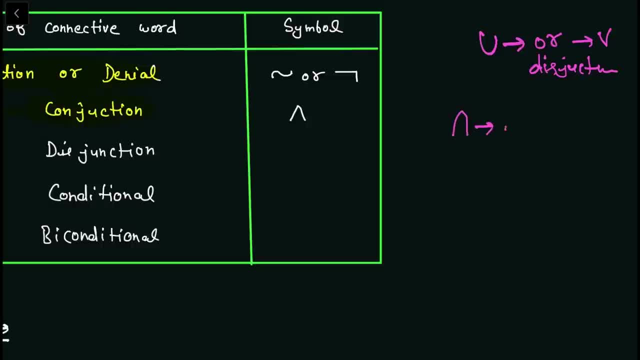 ok join is called disjunction 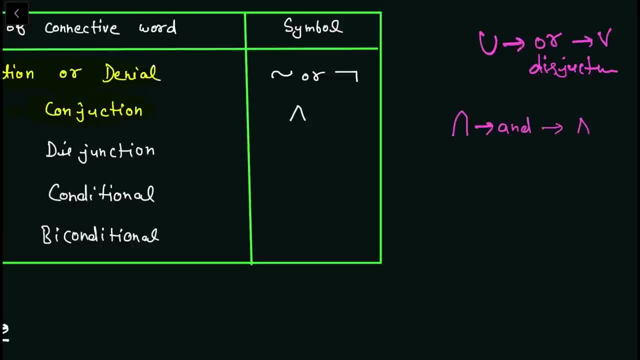 ok we use intersection for end 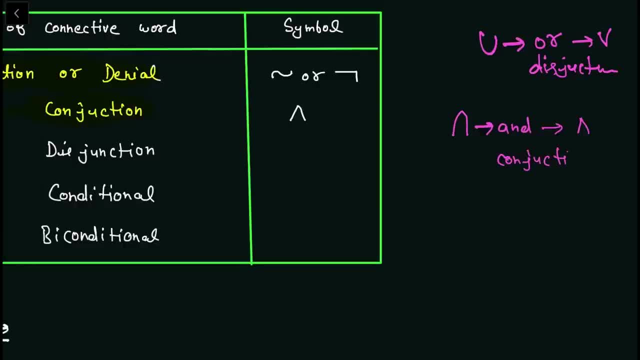 and for end we use meet operation and meet is called conjunction so in this way you will remember them ok 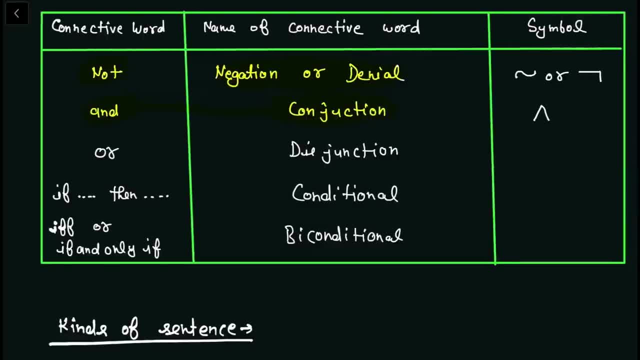 so this meet operation we will name it as conjunction in fourth module and if there is word end between two statement then we can combine it with conjunction 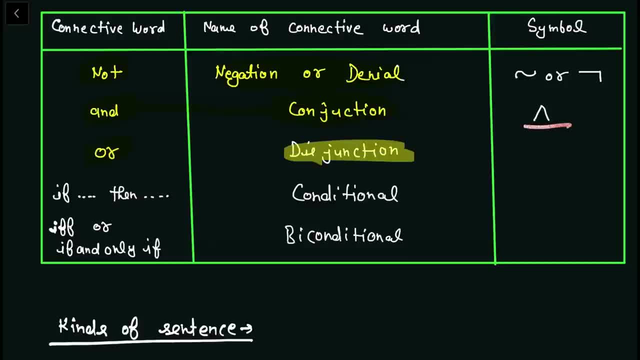 then comes our or operation or operation we call it disjunction and for disjunction we use 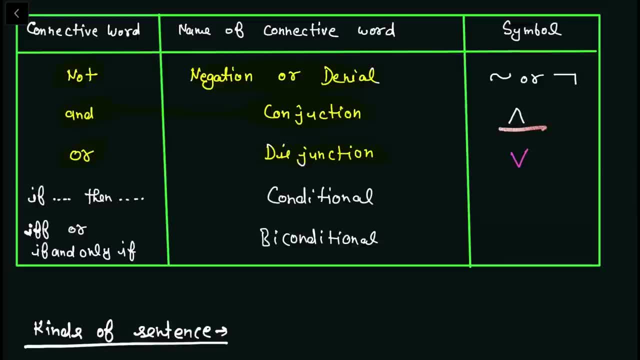 join for disjunction we will use 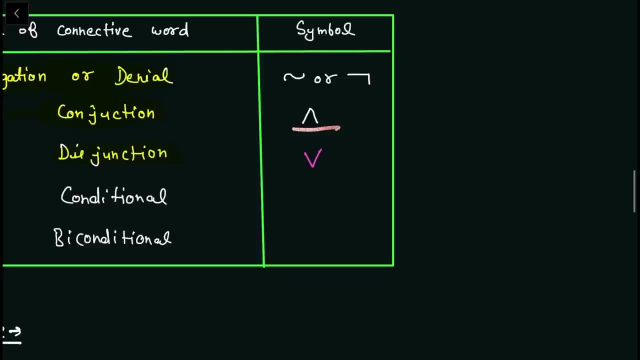 join if there is word end between two sentence or two statement 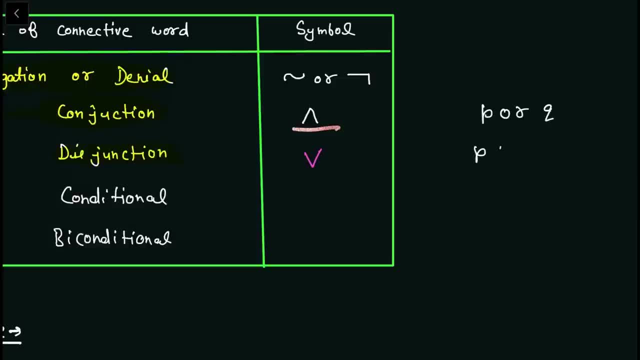 then we can use join which we call disjunction like p and q is written somewhere so it means 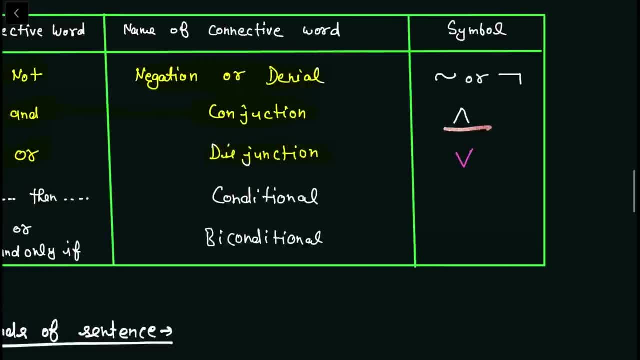 p disjunction q if there is word end between two statement 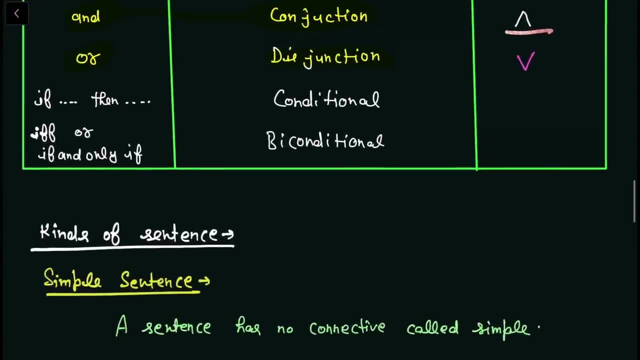 then we use it ok this is its notation 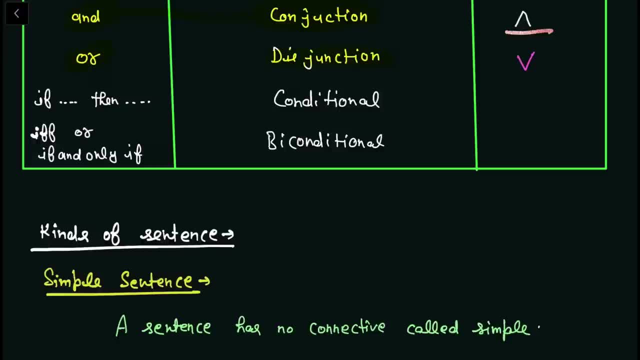 then comes our if then statement if then statement 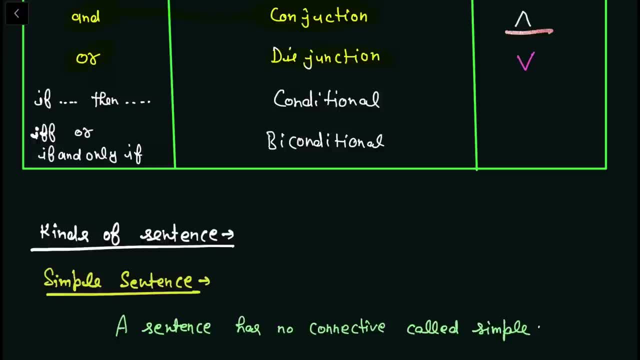 which we call conditional statement if some value will be then some value will be like if p then q we call it conditional statement 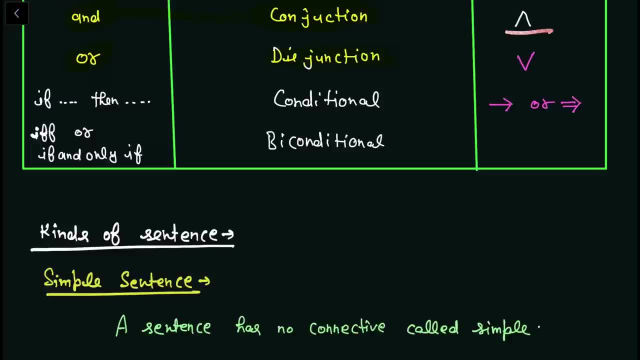 and we use it with two symbol either with simple arrow or with implies or we use it with implies 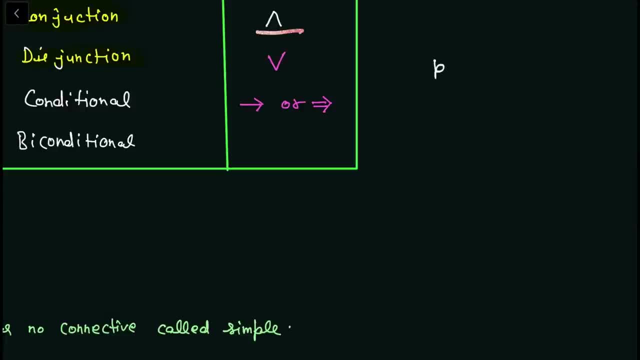 ok for example i take a p statement i said 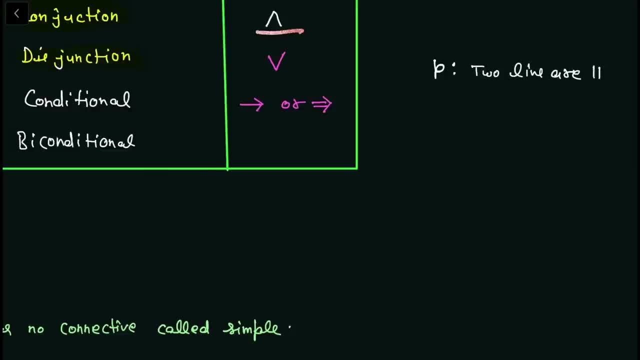 two lines two lines are parallel i said in p statement 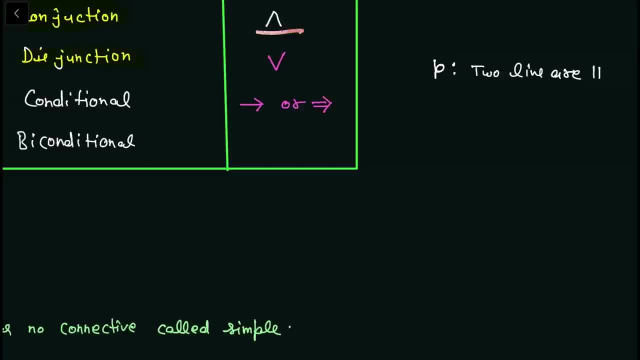 that two lines are parallel and then i said then they do not intersect 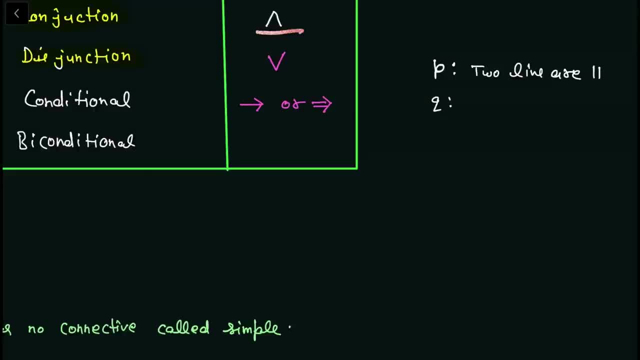 two lines are parallel do not intersect 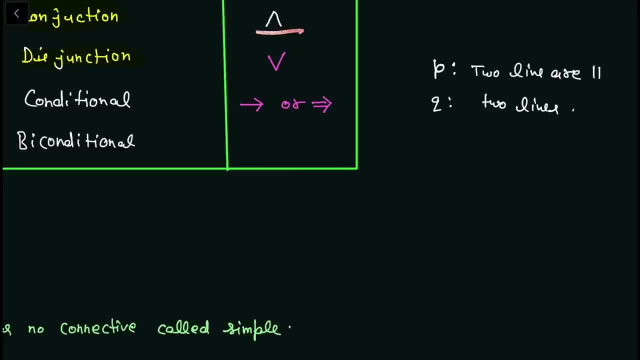 so i called q two lines do not intersect 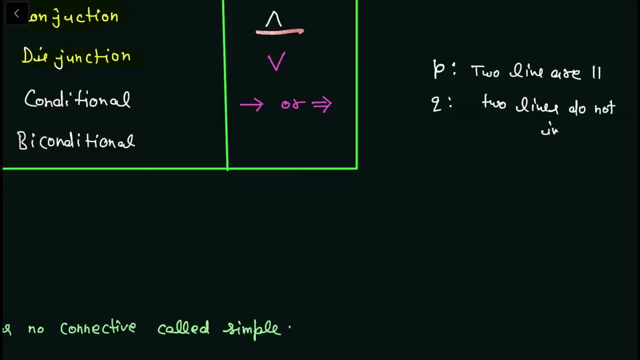 two lines do not intersect means it won't cut when it is parallel 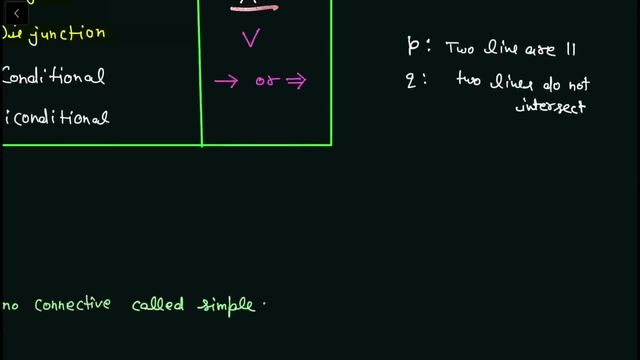 this is simple so two lines are parallel then they 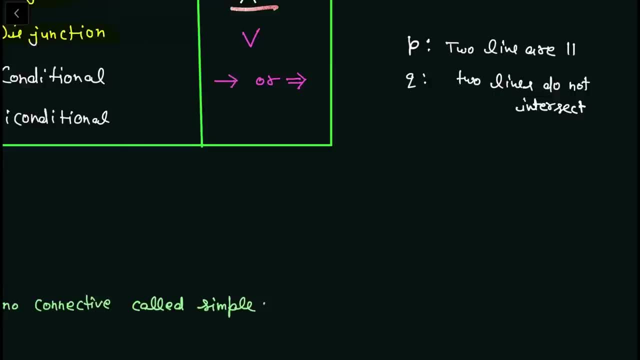 do not intersect so we called p statement 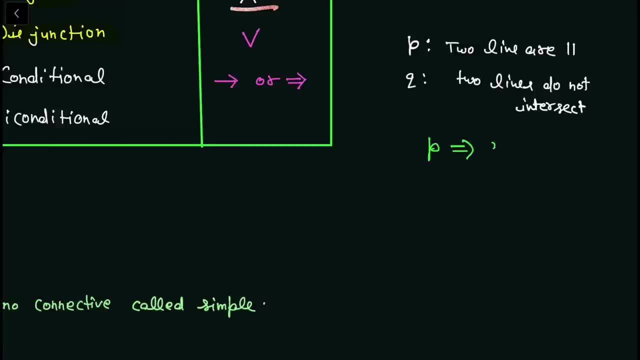 that two lines are parallel q is also uncle we called p imply q 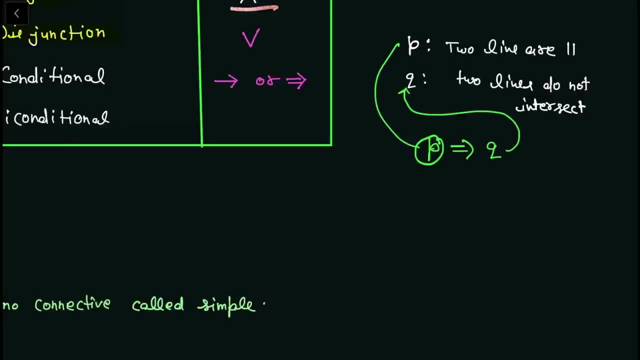 If two lines are parallel, then it will never intersect, implies Q, this implies two lines do not intersect. 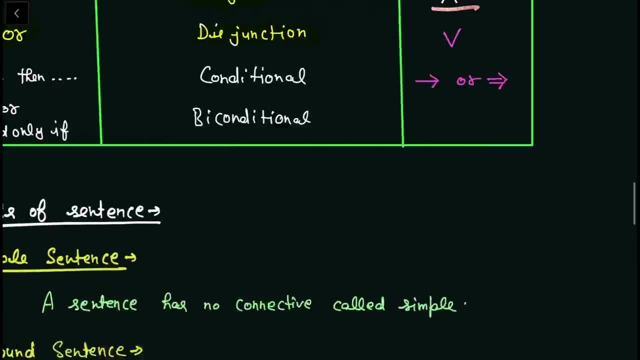 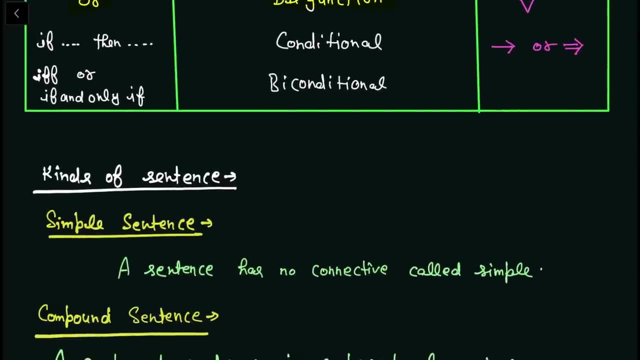 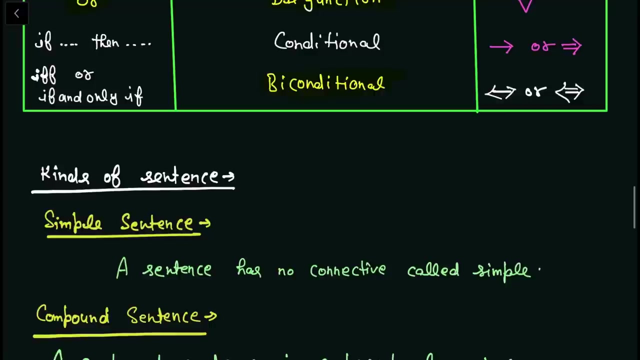 So, this is our conditional statement, which we use with the sign of implies. We can combine two statements with this, we can make it in the form of compound sentence. Then in the last comes our if and only if, which we call a bi-conditional statement, implies and if and only if, you have read in the second module of group theory, in the first module, for if and only if, either we use this kind of arrow or we use this kind of arrow, if and only if, both parts are there, means if there is a P statement, then Q will happen, if there is a Q, then P will happen, conversely, they are for each other, so we use this kind of arrow. 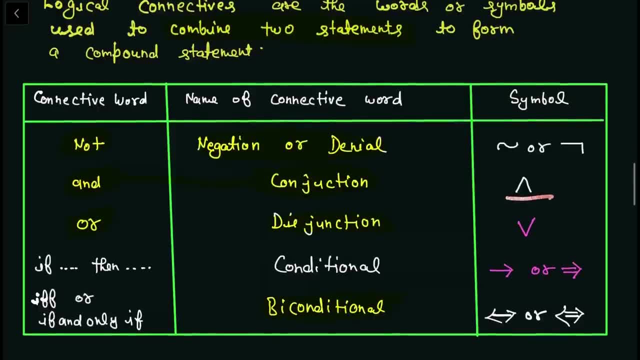 We call it a bi-conditional statement, and with this we can combine two sentences or two statement prepositions. 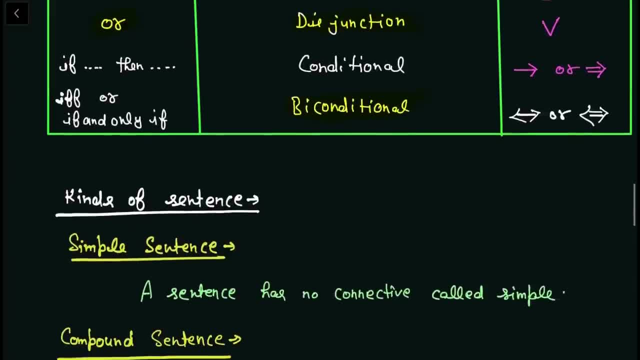 So, mainly, we will work on only five operations in module 4, which I have told you. 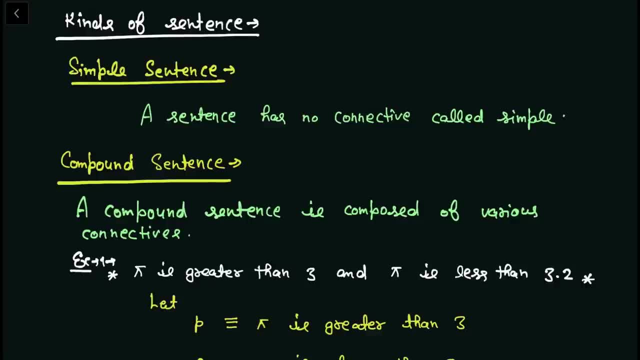 Kinds of sentence, in the kinds of sentence, first of all, let's talk about the simple sentence, what is a simple sentence, if there is no connectiveness in the sentence, means if there is no connection, if there is no operation used, then it will work as a simple sentence, a sentence has no connective, called simple sentence. So, in the sentence in which there is no connective, there is no connection, then we say that it is our simple sentence. 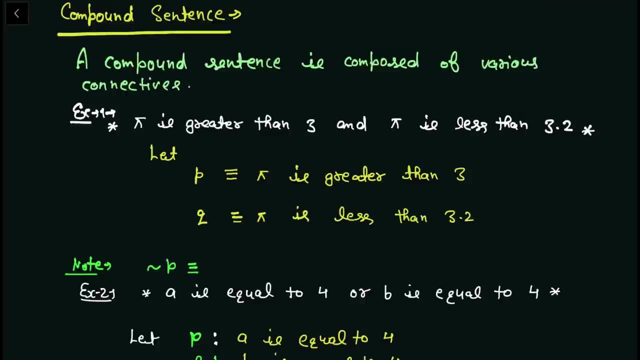 Then comes our compound sentence, compound sentence is a simple thing, in this, there will be at least two statements, and between two statements, there will be some connective, or it will be a conjunction. 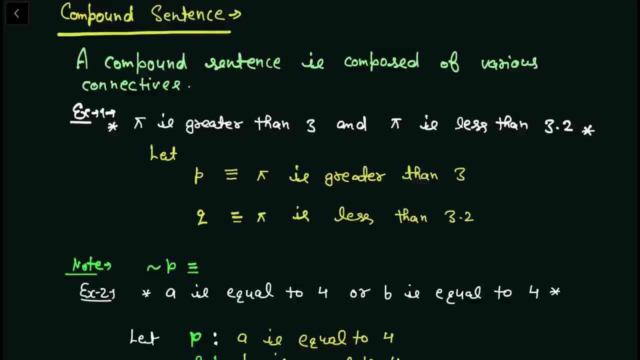 So, there will be a conjunction, there will be a disjunction, there will be a negation, there will be a conditional, and there will be a bi-conditional. So, there will be some connection in them, so that will make our compound sentence. 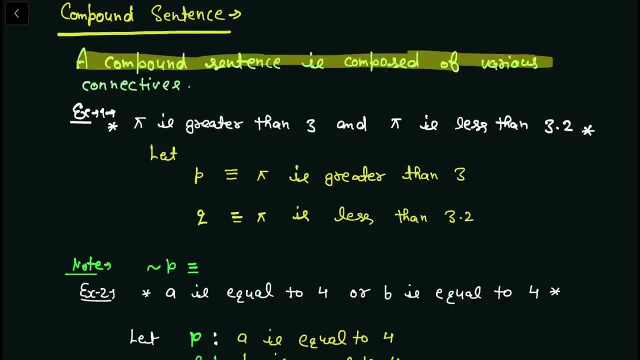 A compound sentence is composed of various connectives, we compose it with various connectives, we combine it, so that is our combined sentence, which we call compound sentence. 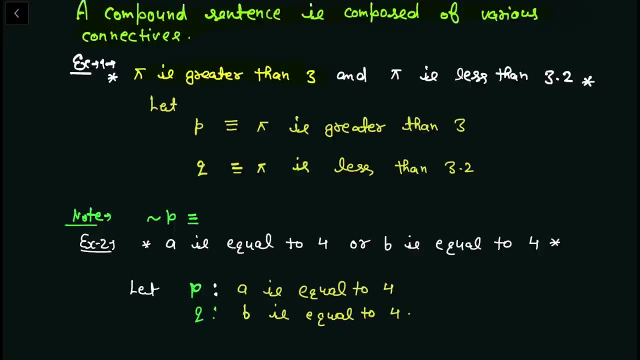 For example, we took the same example above, that pi is greater than 3. And pi is less than 3.2. So, here I named the p sentence that pi is greater than 3, we named it as p sentence. We named q as pi is less than 3.2. Because here you can see that the end word has been used, so you can call it a simple thing, p and q. p and q, for the end we will use conjunction. 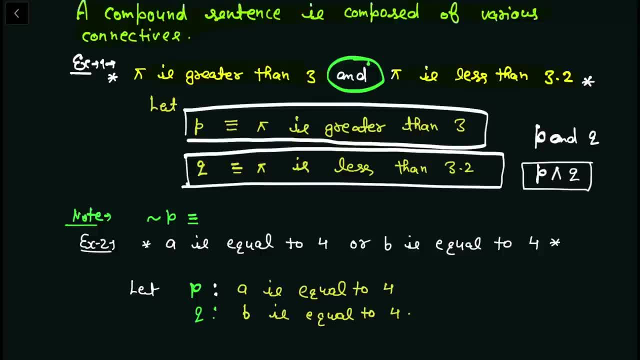 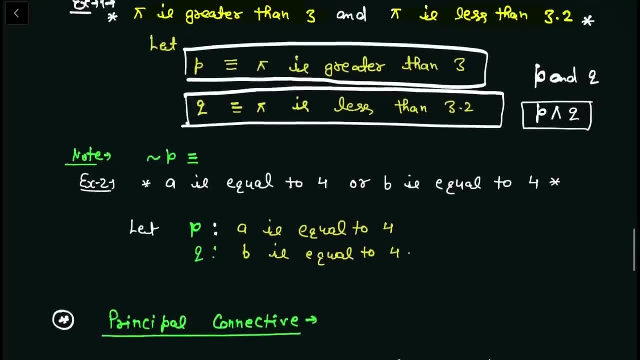 p and q. So, the compound sentence made here is made of conjunction, which you call meet. p meet q, means p conjunction q. So, this is our compound sentence, we have made it by combining two sentences. 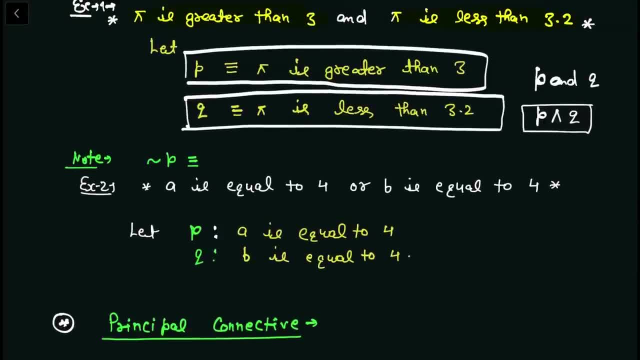 And what is the operation used? Conjunction, which you call meet. 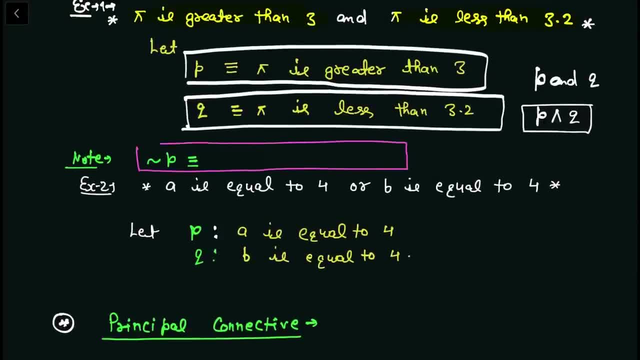 If we take out the negation of p here, then the negation of p is very simple. Here you have said that p is greater than 3. What did you say there? p is greater than 3. 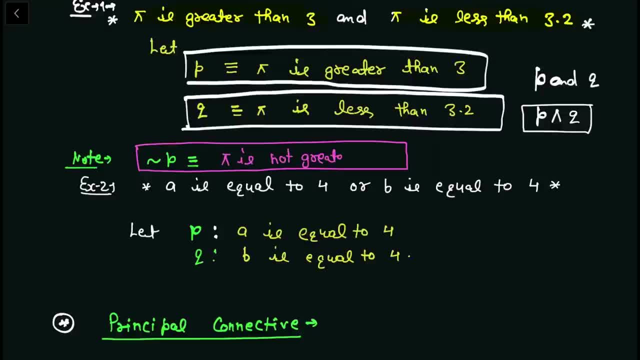 So, what will be its negation? p is not greater than 3. This is a simple thing, it will be reversed. 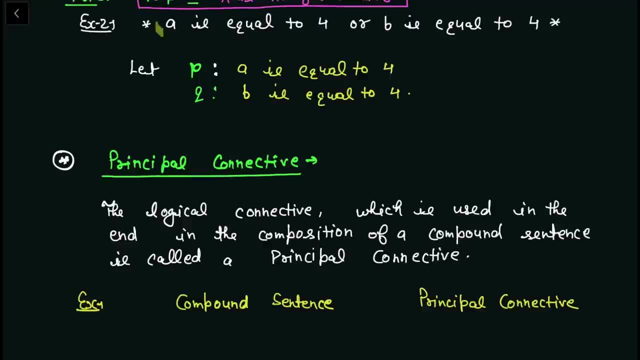 Then, the second compound sentence example, that if a is equal to 4 and b is equal to 4. So, we named both the sentences here. I gave the name of p to one. a is equal to 4. I gave the name of q to one. It is of statement. 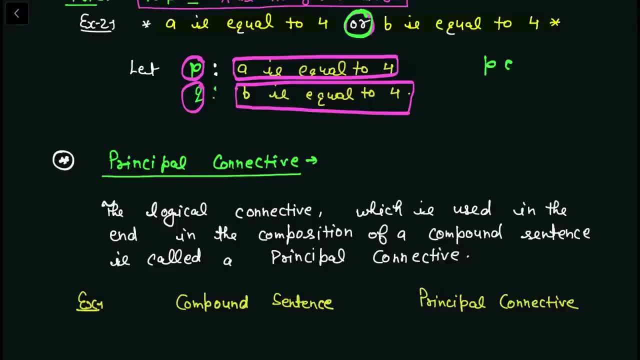 And it is called b is equal to 4. Because more words have been used in it. 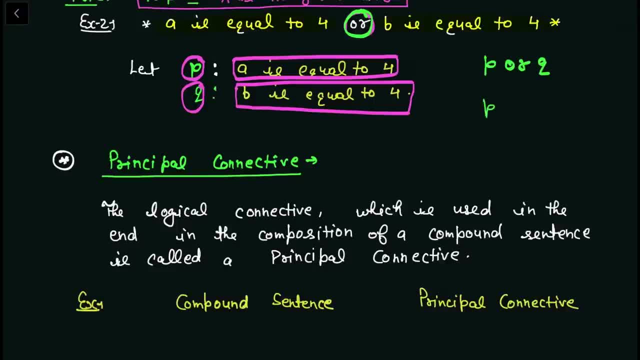 Because of this more word, p and q will be made here. How will the combination of both be made? From p and q. 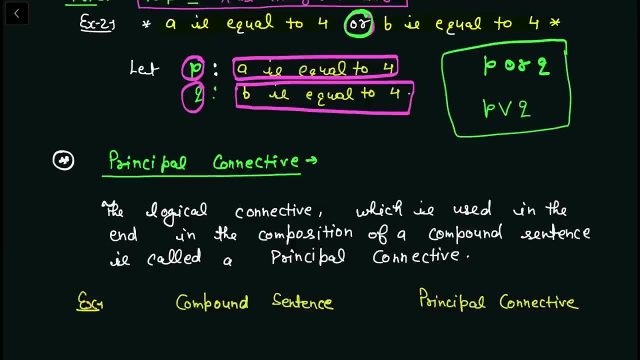 And for more we use disjunction, means join. What do we use for more? Disjunction, means join. So, this is also our compound sentence. Compound statement will be made. 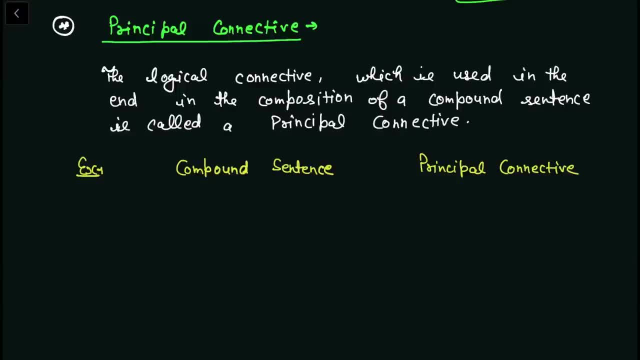 Then, let's talk about principle connectives. Okay. 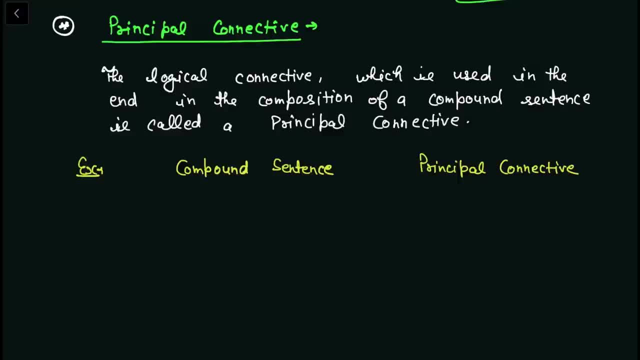 See, if you have a compound sentence. So, in it, the 5 operations that I have told, 2, 3, 4 out of 5, how many operations can be used? 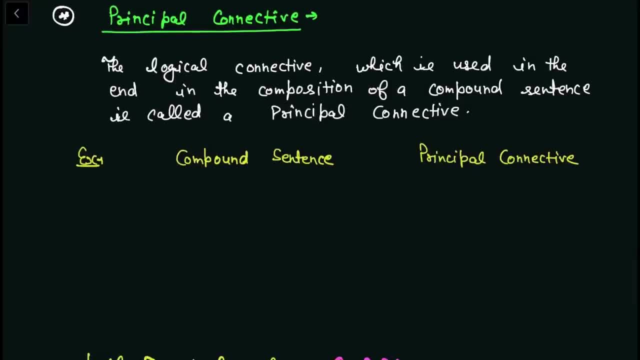 So, in it, understand the principle connectives. What are the principle connectives? Principle means the main. From which your result comes out in the last. 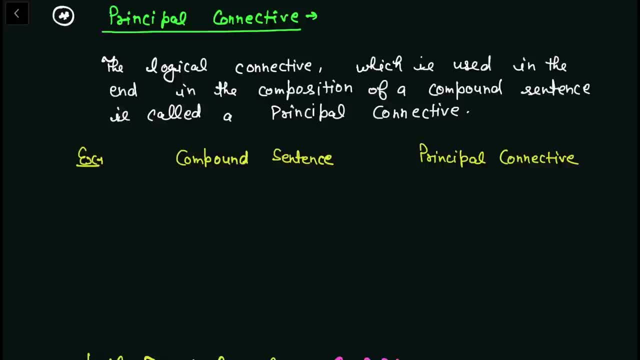 That is called our principle connectives. The logical connectives which is used in the end in the composition of a compound sentence is called principle connectives. Okay. 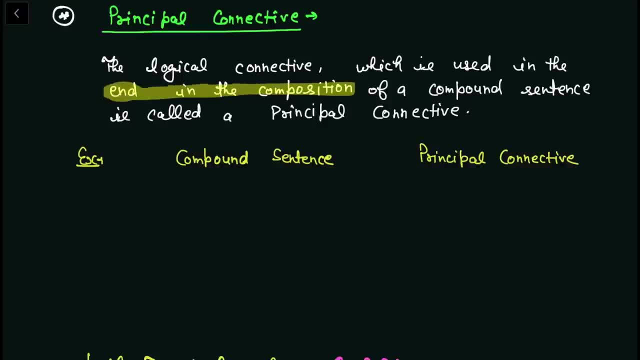 The main operation or connectives that will be used in the last. Whether it is conjunction, disjunction, negation. Okay. Or conditional or bi-conditional. Whatever is used in the last of any compound sentence. 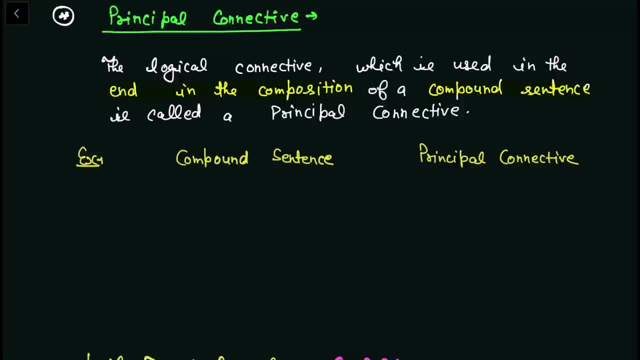 That is our principle connectives. 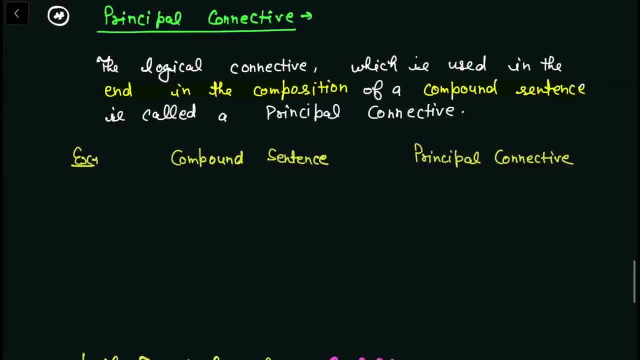 For example, I took a compound sentence. How did I take a compound sentence? 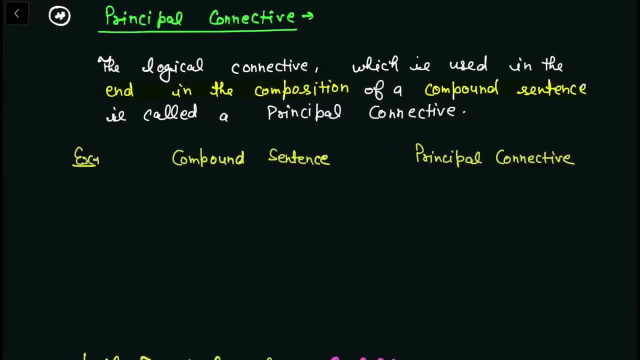 On one side, I wrote compound sentence. On the other side, I wrote principle connectives. So, on one side, I made a compound sentence that P conjunction Q implies R. So, this is my complete compound sentence. 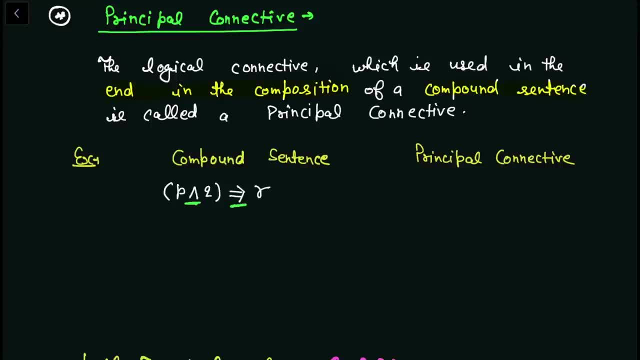 In it, 2 operations have been used. One is conjunction which is used for the end. One is implies. 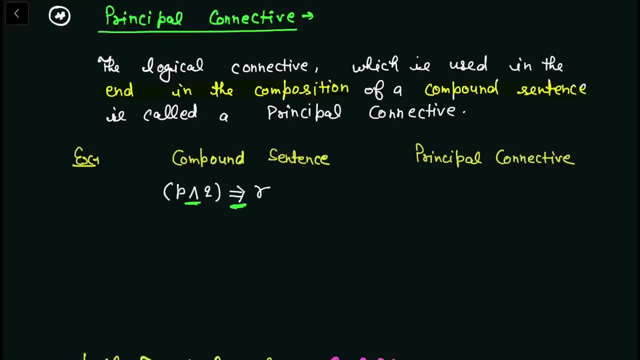 That is, conditional statement. So, what will we do first? 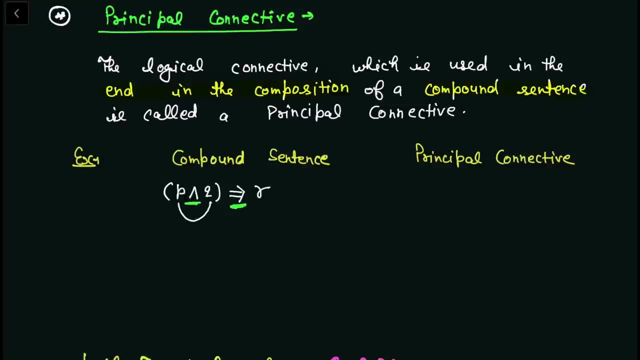 We will have P, Q, R, 3 propositions and statements. First, what will we take out of P and Q? We will take out conjunction. Then, after taking out conjunction of P and Q, one of our new statement will be made. Right? From whom do we have to do that statement's implies? From R. That means, from whom do we have to take out its conditional? From R. And in the last, which operation will be performed? Which will be ours? It will be implies. 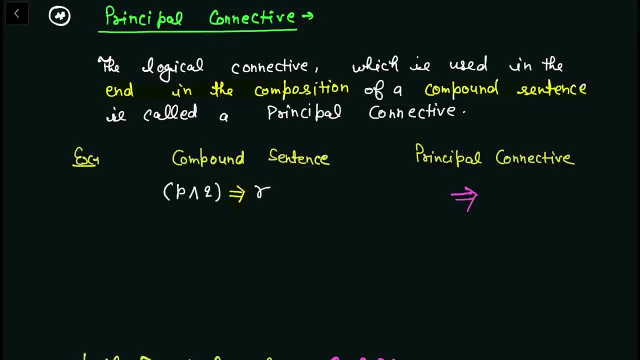 And this implies will work for principle connectives. Similarly, I took a compound statement that R implies P join P if and only if Q. Right? To solve this also, what will you do? First, we will solve this bracket. 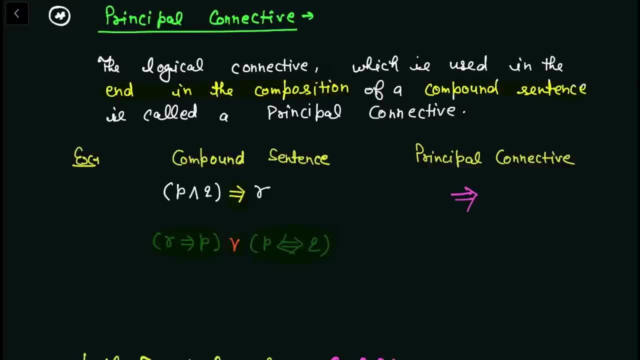 Then, we will solve this bracket. In the last, we will use this join operation. 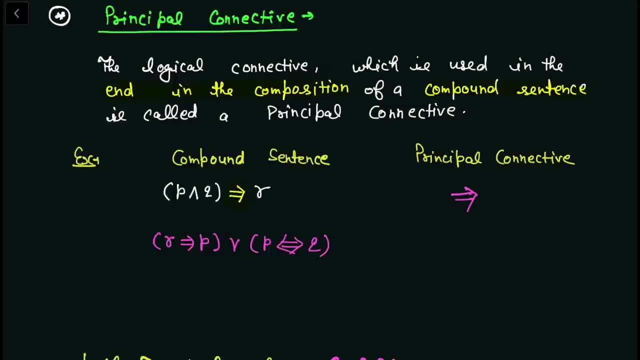 So, in the last, which is performed in the end. Which is performed in the operation. That only works for our principle connectives. 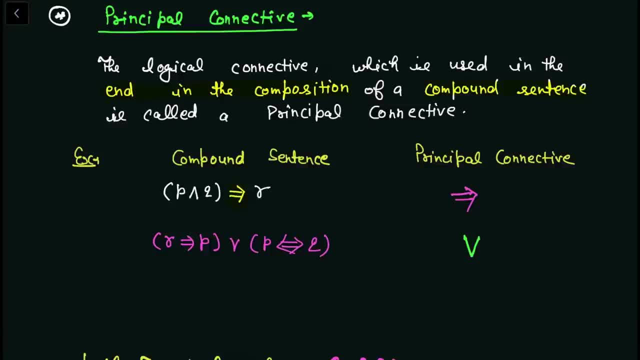 So, here the principle connectives are joined. Which is used in the end. 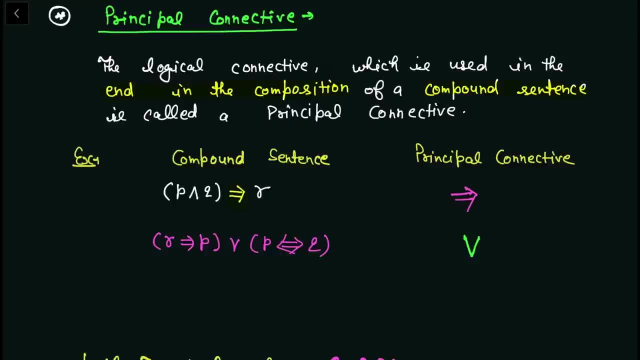 So, I told you about operations. Right? And how we can compound this statement. 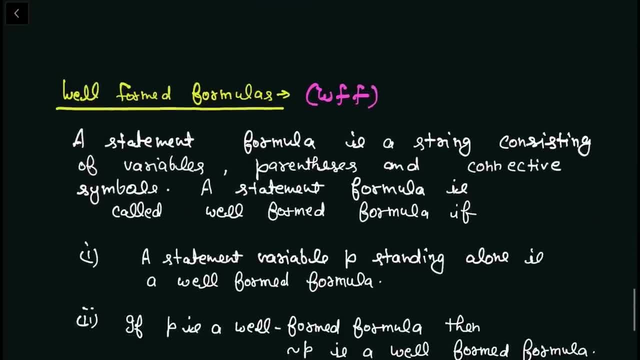 Can tell simple statement. Or conjunction, dejection, negation. What is this? 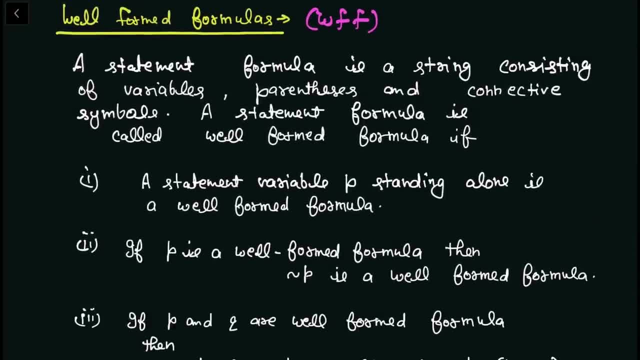 Now, while using all these, we can call any compound statement as well-formed formula. Right? Well-formed formula. 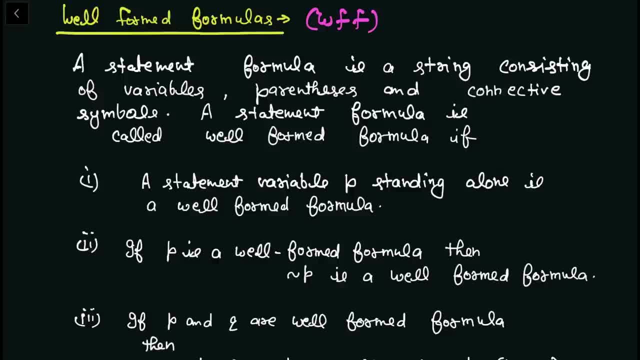 What is its definition? This is often asked in the exam in two numbers. Only definition will be asked. 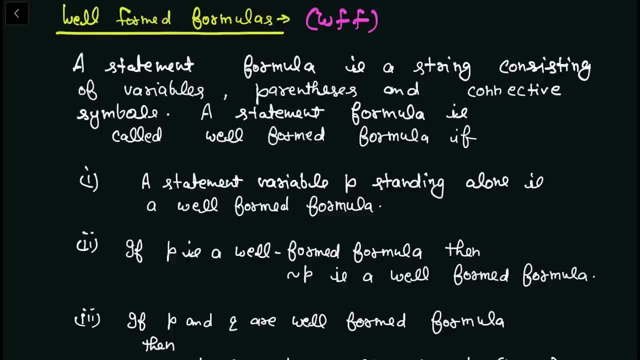 So, what is well-formed formula? A statement formula is a string consisting of variables. In which propositional variables will be there. PQR, parenthesis, brackets will be there. And connective symbols. And along with that, symbols will be there. Like conjunction, dejection, negation. Or conditional or bi-conditional. Right? 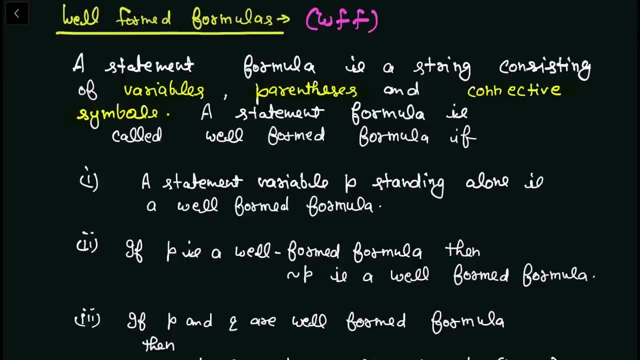 So, any compound sentence in which there will be PQR variables, brackets and connective symbols. 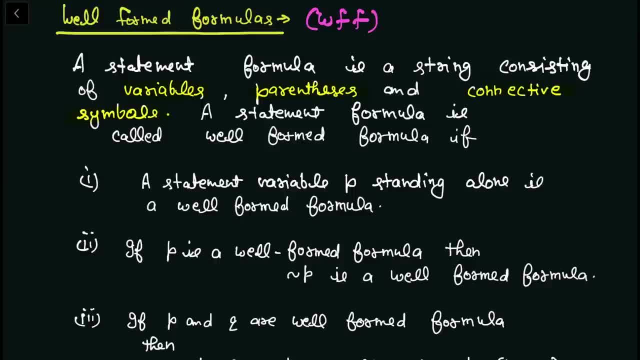 So, we can call it as well-formed. We can say that our statement here. This proposition is made. This is our well-formed. It is made very well. But when will we say? 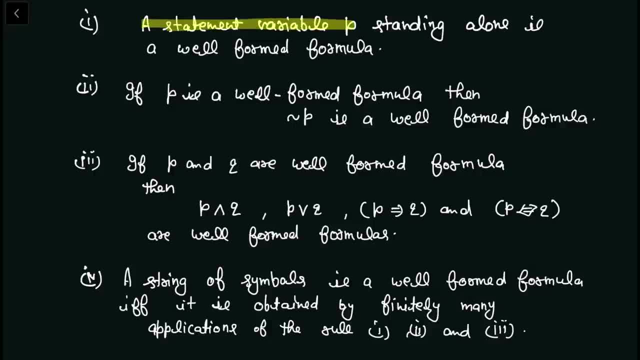 We can say this only if it satisfies some conditions. First condition. That A statement variable P standing alone is a well-formed formula. 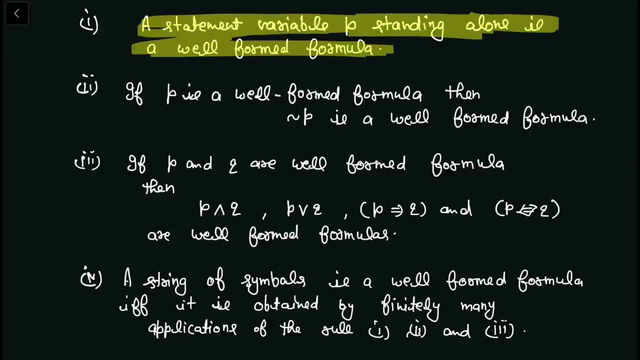 Whatever we have defined as P variable. It should be well-formed. Right? What should that be? It should be made very well. 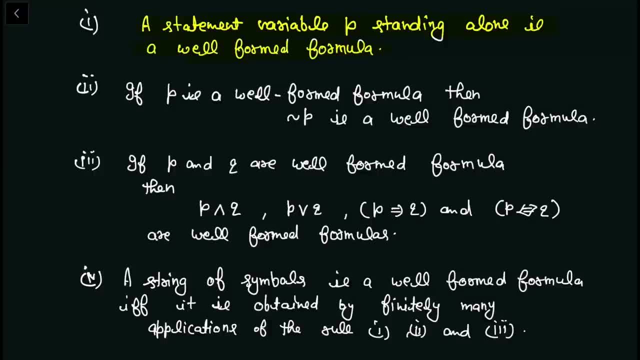 And we call it as well-formed formula. If P is our well-formed. Right? So, if P is our well-formed. 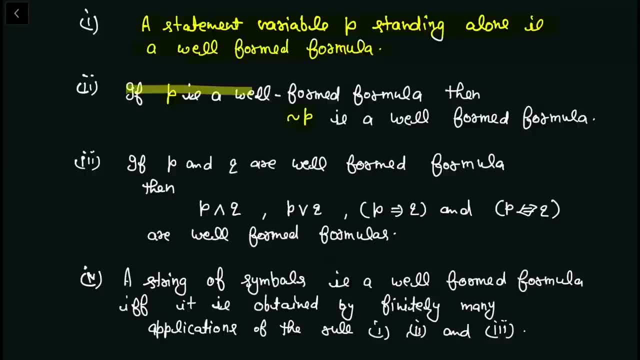 So, its negation. It is simple. It will also be well-formed. It will come in well-formed. So, we have written the second condition. If P is well-formed formula. Then the negation of P should also be our well-formed formula. Second condition. For such Q variable. 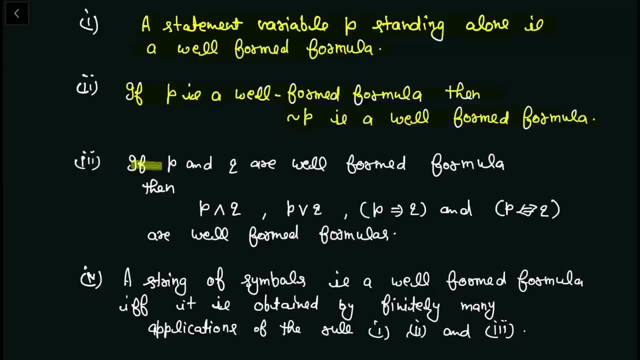 For R variable. If it is used in it. Then PQR will be a condition for all. Then if you have told both P and Q as well-formed. 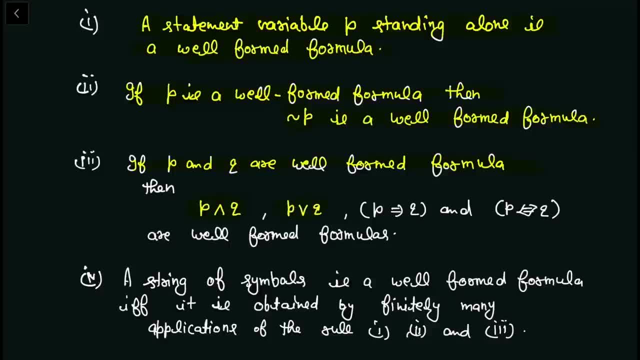 Then it is a simple thing. You remove their join. That is, you remove their conjunction. You remove their dejection. Or you remove their P conditional. 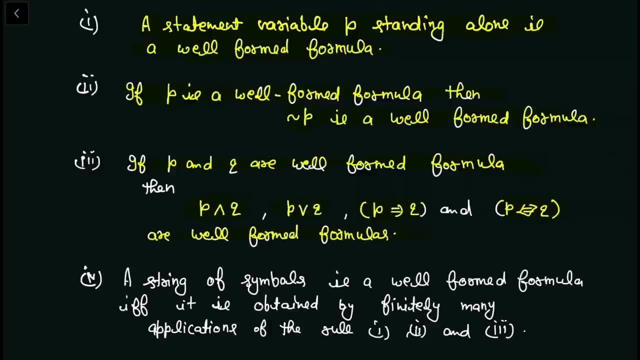 Why remove P conditional? Or why remove P biconditional? Right? 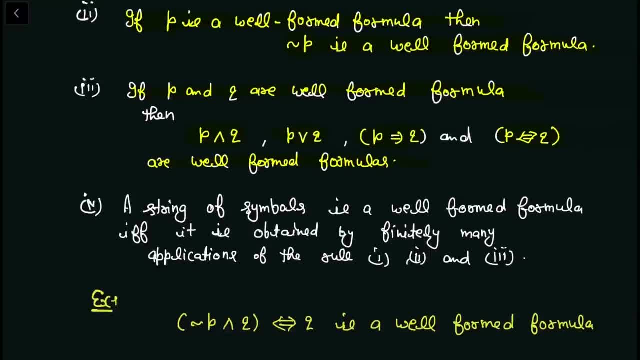 So, all of them will also be well-formed formula. And by using all of them. Our finally compound statement will be derived. 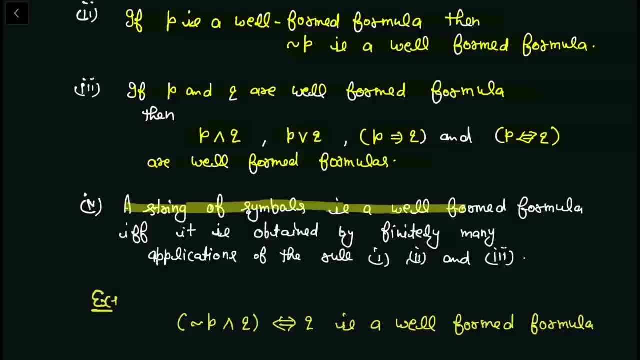 It is a simple thing. It will also go in our well-formed. I have written in the last. String of symbols is a well-formed formula. 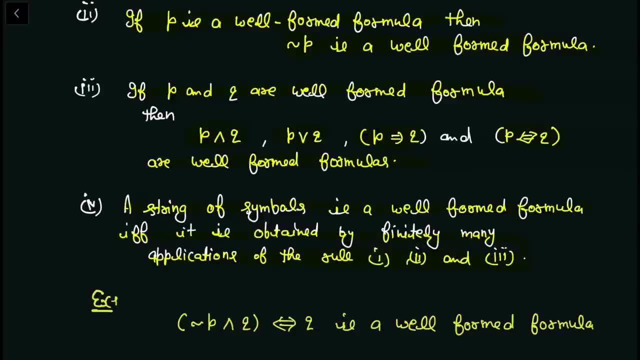 If and only if. It is obtained by finitely many application of the rule 1, 2, 3. On which I have told 1, 2, 3 rule. If we use them. 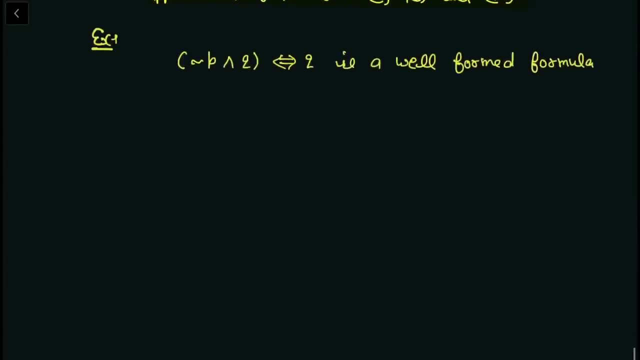 If we make a compound statement by using them. Then it will also be told in our well-formed. Like for example. Negation P. 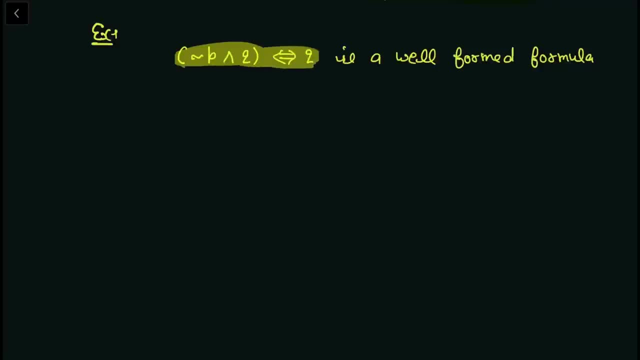 Conjunction Q. And biconditional Q. This will be our well-formed formula. If your P is well-formed formula. Q is our well-formed. Then whatever compound statement will be made from them. It will also go in the well-formed. Okay. So, today's lecture.